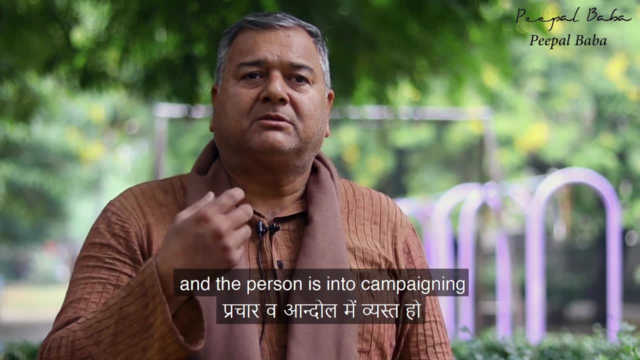 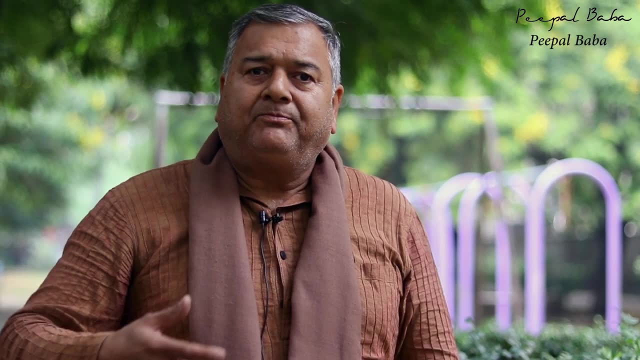 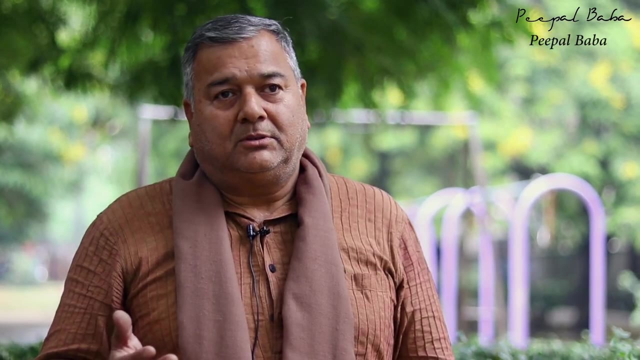 any work on the ground, but the person is into activism and the person is into campaigning. the organization is totally into advocacy. that itself is very important. That is also very important because you need to create a buzz so that the ground is laid for those. 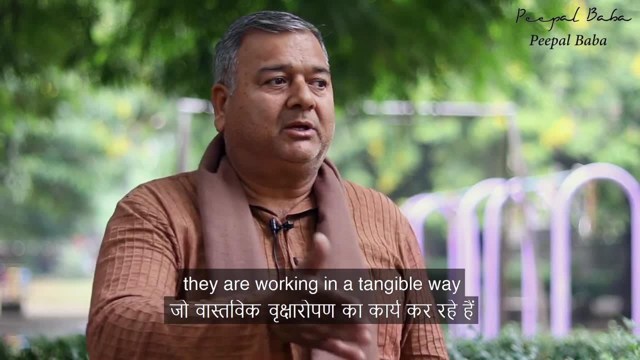 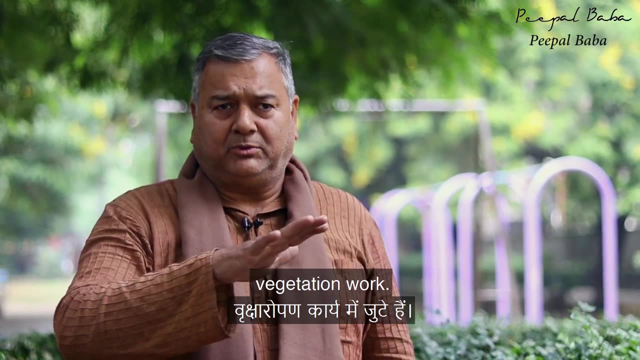 people who are working on the grassroots. They are working on the ground, they are working in a tangible way, producing results. Like we are totally into hard core, into plantation work, vegetation work, from small shrubs to big trees. you know we are there to create. 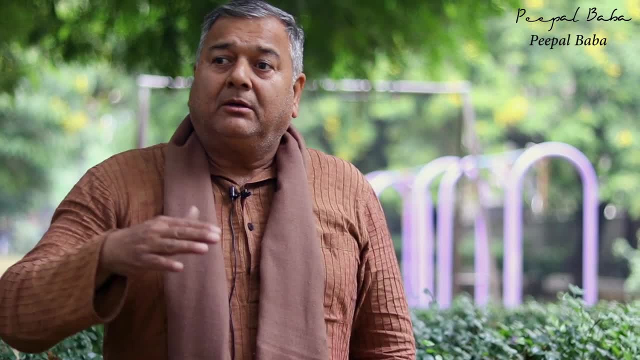 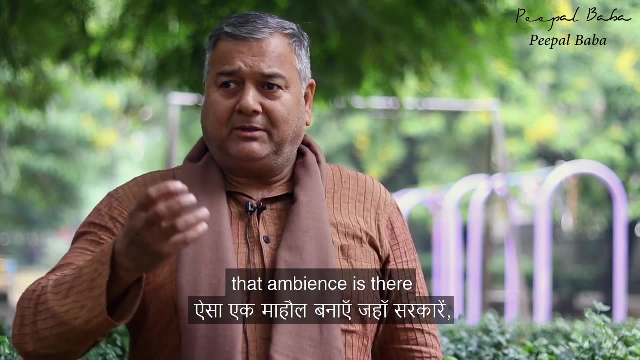 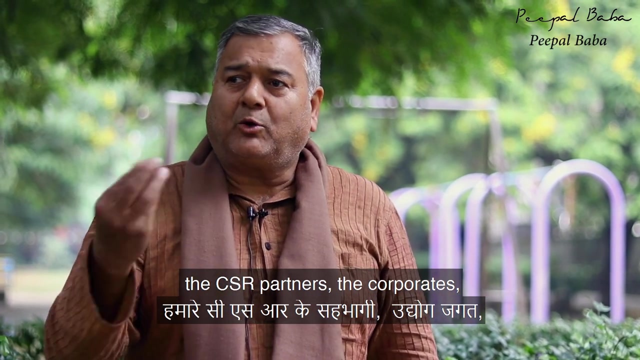 this thing. But this cannot be done till the time, you know, the buzz is created, people create that environment, People create that ecosystem. That ambience is there where the government departments, the authorities, the CSR partners, the corporates, they are not aware. So all that I am trying, 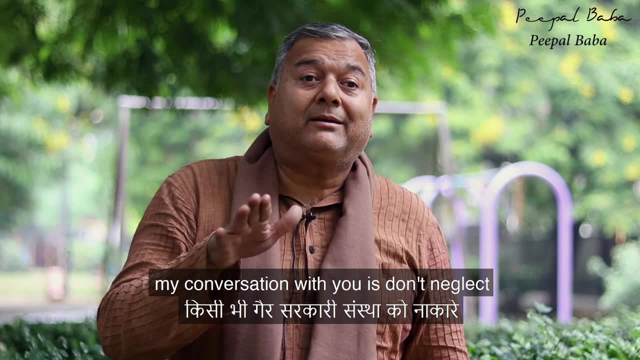 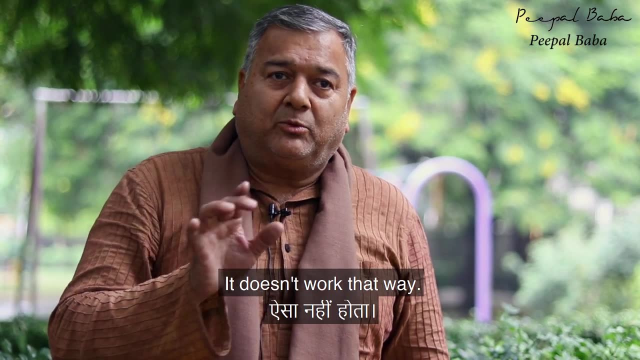 to say in my conversation with you is: don't neglect and don't say that this NGO is not doing good work or that group is not doing good work. It doesn't work that way. Everybody has a role to play. Everyone has a role to play. 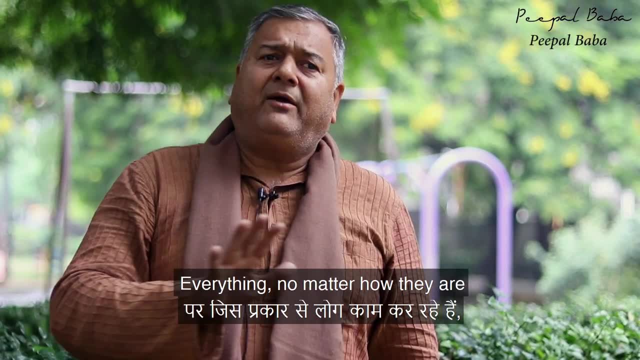 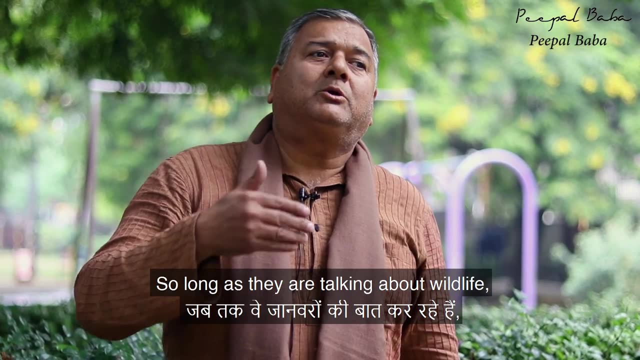 Right, There are small players, there are big players, everything, no matter how they are working, with whatever intention they are working, so long as they are talking about wildlife, they are talking about environment, they are talking about rivers, they are talking about. 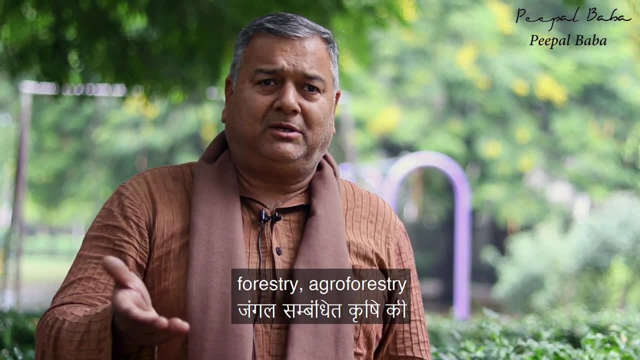 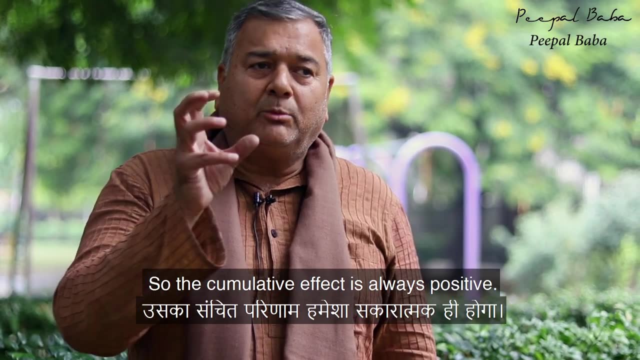 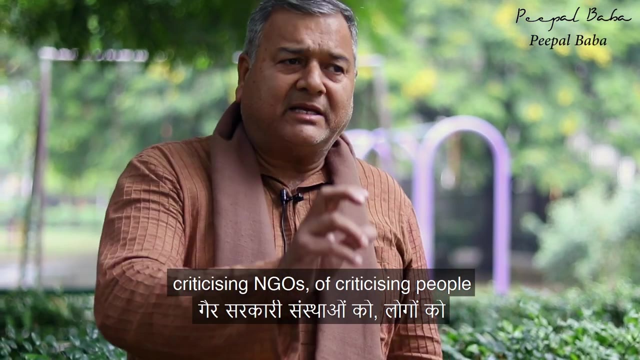 farming, agriculture, forestry, agroforestry, social forestry. We need them. It's teamwork, It's total teamwork, So the cumulative effect is always positive. So do not get into this race of criticizing NGOs, of criticizing NGOs. Do not get into this race of criticizing NGOs, of criticizing people, of criticizing groups. 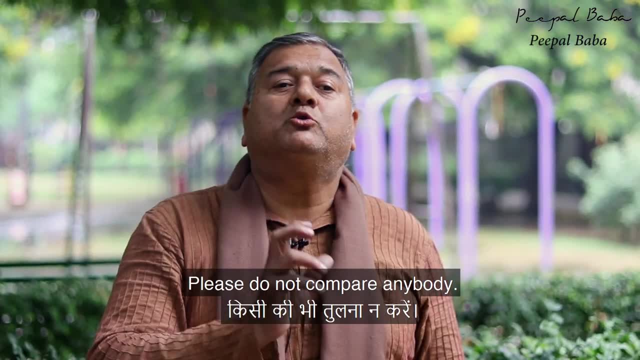 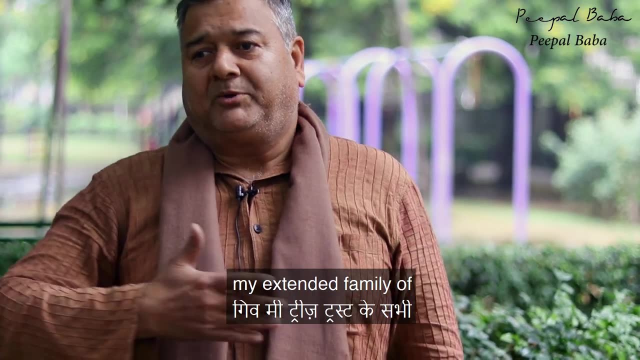 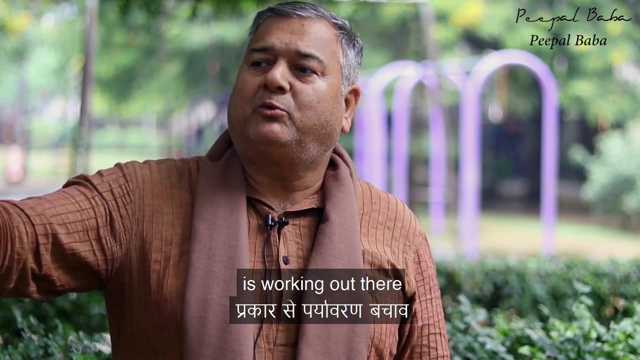 of people, that they are doing good work and bad work. Please do not compare anybody. This is what I want to say. My message to all my volunteers, my teammates, my extended family of GiveMeTreesTrust is that everyone, everyone, whoever is working out there in this line of 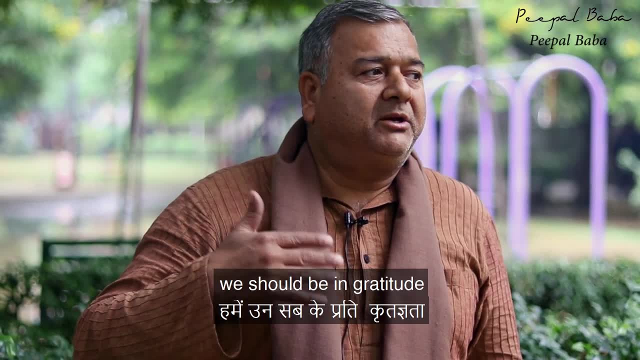 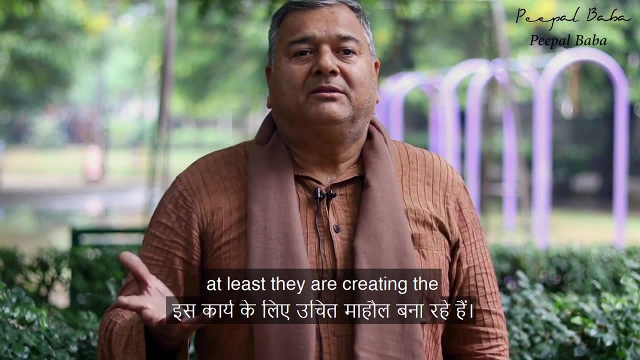 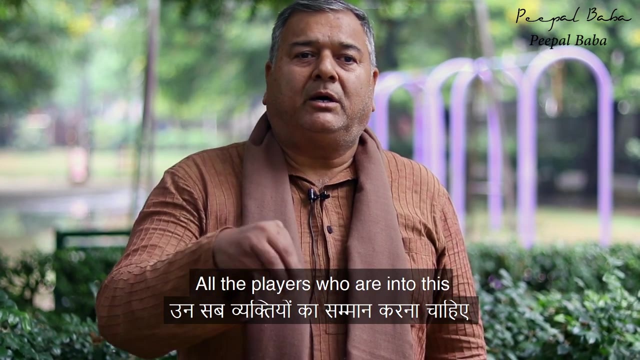 work is. we should be, we should be in gratitude of them and we should be grateful to them that at least they are creating the buzz, at least they are creating the right type of ecosystem. So everybody has a role to play. We should respect everybody, All the players who are.